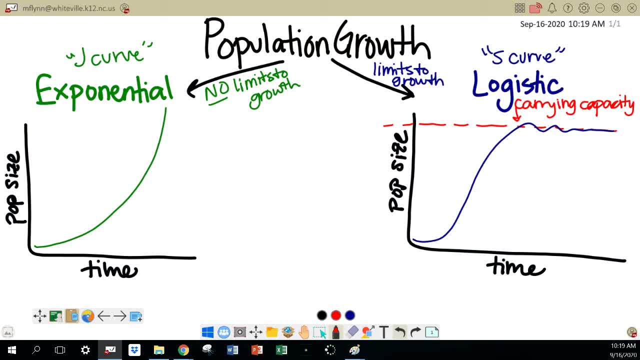 so it stays consistent in size because of limited resources of some kind. So it could be limited food, limited shelter or limited water, Or if the population is too big, it could be that they're really prone to diseases, things like that. 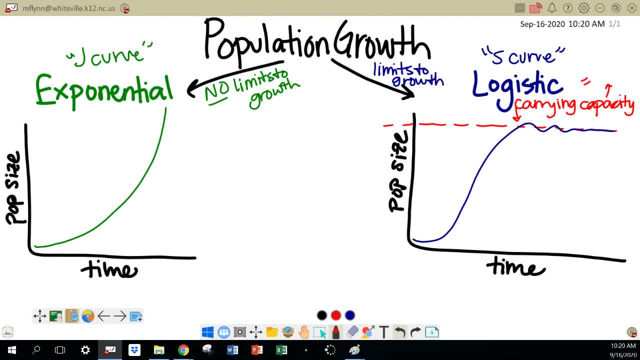 So carrying capacity, that is your limit Due to lack of resources. Okay, so that's the limit due to lack of resources, okay, So that term is really, really, really, really, really important. So the reason why there is a limit in logistic growth is because of that: carrying capacity, okay. 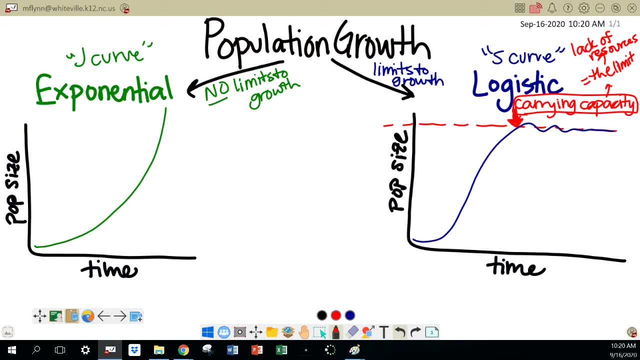 So that is that red dotted line, So that's where it levels off. So notice, with the exponential, it does not do that, So it continues to grow faster and faster. Okay, so it'll keep growing. It'll keep doing that forever, according to that model. 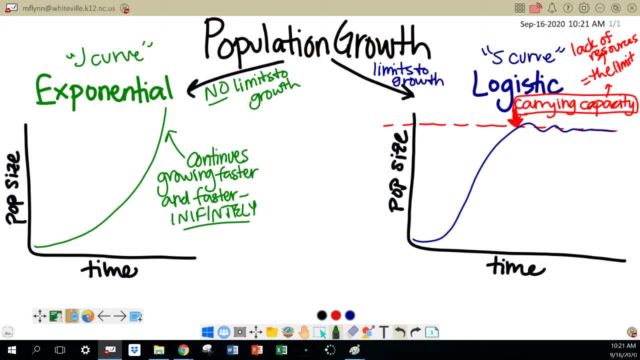 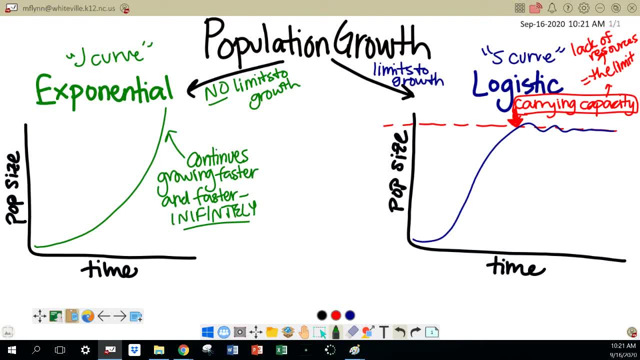 that totally covers a blanket over all of the trees, and all that on the side of the road. it is basically growing exponentially. It's growing as fast as it can because there's nothing at this point that's limiting its growth, Whereas if you have something like 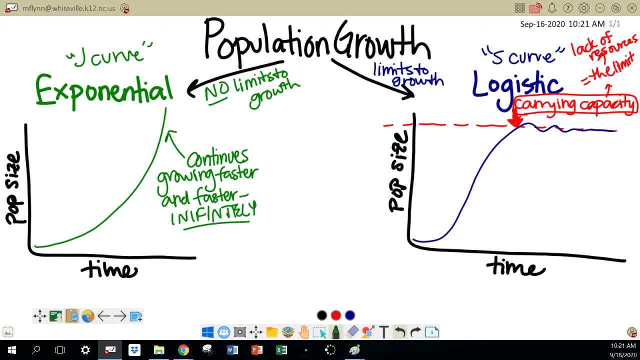 oh, I don't know, a certain number of mice in an area. There might only be a certain number of places they can burrow or whatever. So they would start leveling off because at some point they would run out of shelter. So the note I wanna make here: 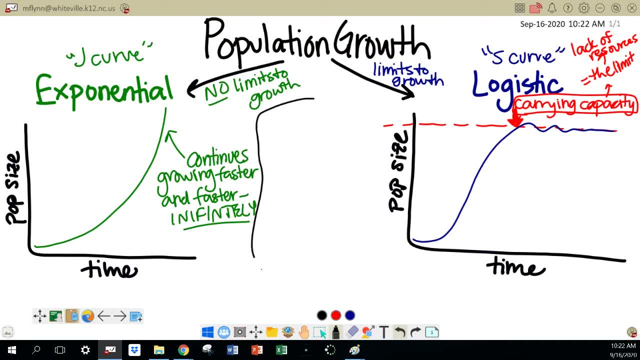 about the real difference between this. I'm gonna make a little box here. All right, so when a population first colonizes an area, it grows exponentially. Okay, so it grows exponentially. I ran out of room there. That's bothering me. I don't like that. 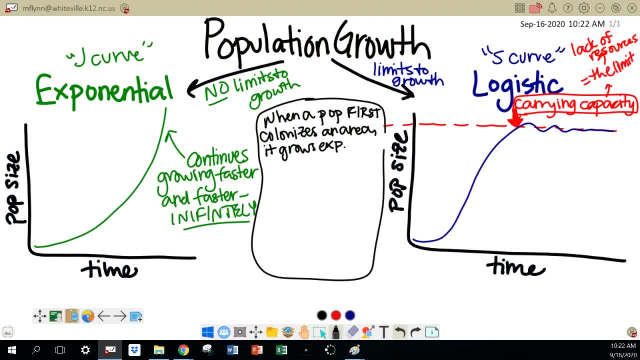 I'm just gonna put EXP: okay, so no limit, Because it hasn't run out of its resources yet. Okay, but then eventually. eventually it's gonna start running out of room, starts getting close and then eventually we're gonna have to move to the carrying capacity limit. 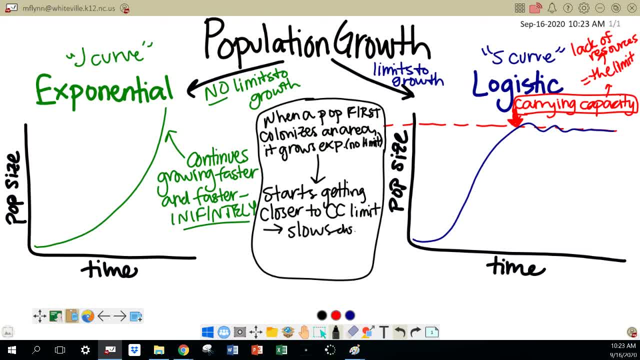 And so then it slows down And levels off. Okay, so the limits there? just to make a list here: Food- Oh, I forgot the food. Yeah, I forgot Food. food shelter, disease, etc. So there's a bunch of things that could cause that limit. 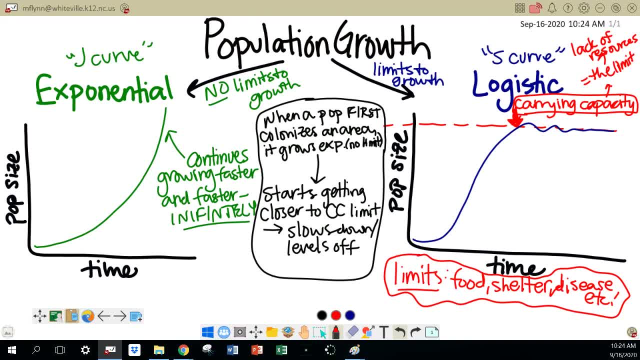 So notice, here it sort of looks like at this point- and I'll use green because it sort of looks exponential right here- So along this point it sort of looks exponential. They're basically nowhere near their limit at that point, so it's going to grow pretty fast. 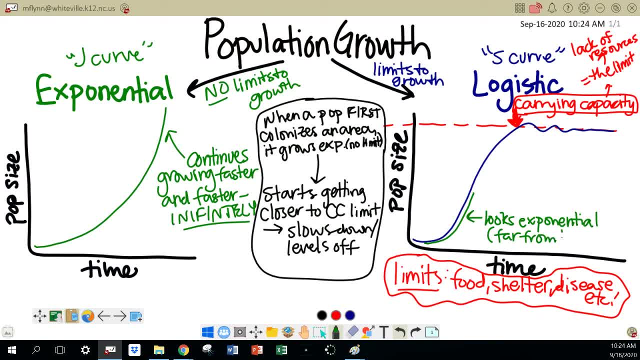 So far from limit, And then it starts to slow down As it approaches limit. and then here it hits the limit and then growth halts. Now notice that it's not going to stop. It's not going to stop.